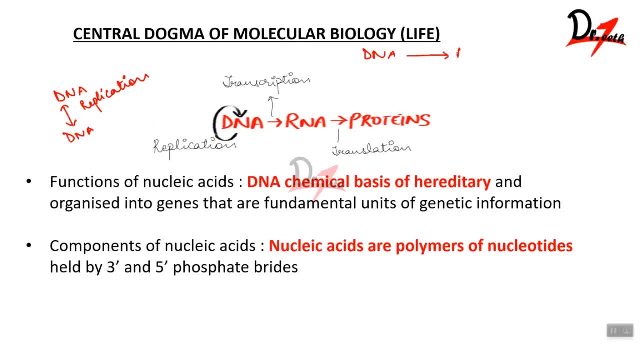 our DNA is converted into RNA, that is, the deoxyribonucleic acid is converted into RNA. then this process is known as transcription- is converted into proteins. we call it as translation. now we all know that the proteins form of the RNA or the DNA. okay, so DNA into DNA is known as the. 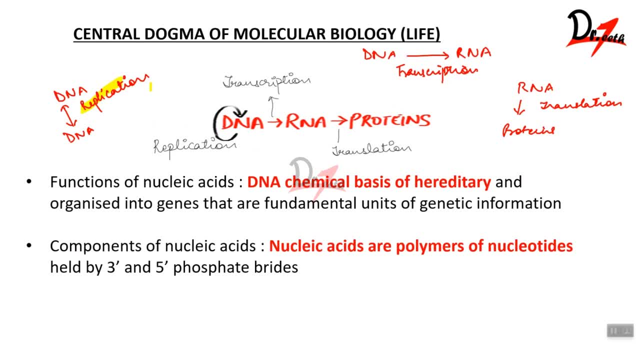 replication. DNA into DNA is replication, DNA into RNA is transcription and RNA into protein is translation. now, what is the function of nucleic acid? now, DNA, chemical basis of hereditary and organized into genes that are fundamental units of genetic information, which means DNA is the chemical basis of. 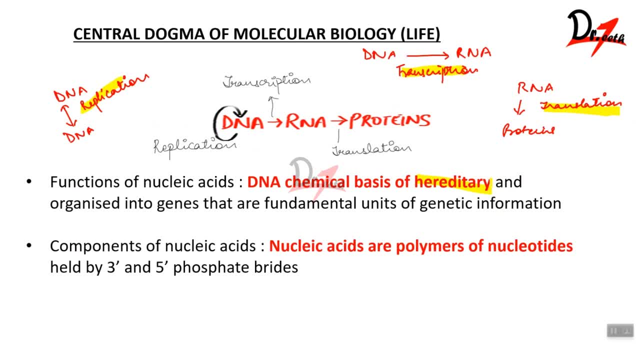 hereditary, like how our genes are transferred from our parents to us and so on, and these are organized into genes. that are the fundamental units of genetic information. now the components of nucleic acids. nucleic acids are basically polymers of nucleotides which are held together by 3 and 5. 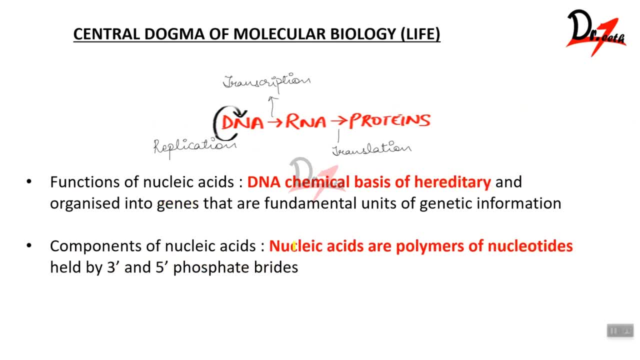 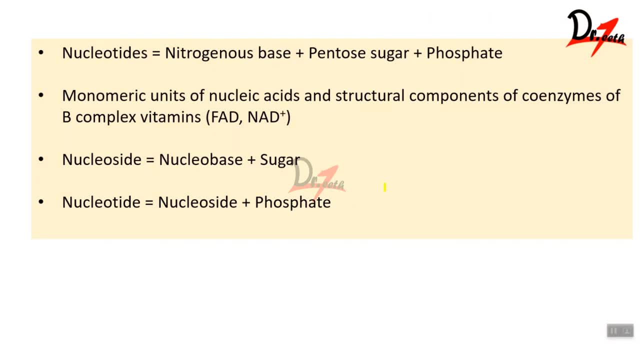 phosphate bridges. we'll be talking next about what we know as nucleotides. now, what are the nucleotides? we have the three main components that form nucleotides. first we have the nitrogenous base, then we have the panto sugar and then we have the phosphate. okay, these are the three different parts. 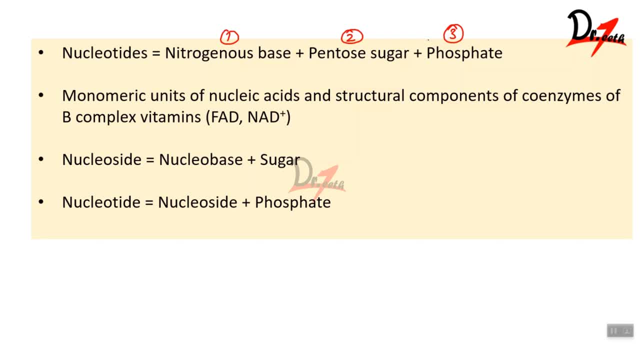 that together combine the nucleotides. now nucleotides are basically known as the monomeric units of nucleic acids and structural components of coenzymes, of beta complex vitamins, like we have the FAD and we have the NAD plus. okay, now the nitrogenous base and panto sugar is together known as nucleoside. we can. 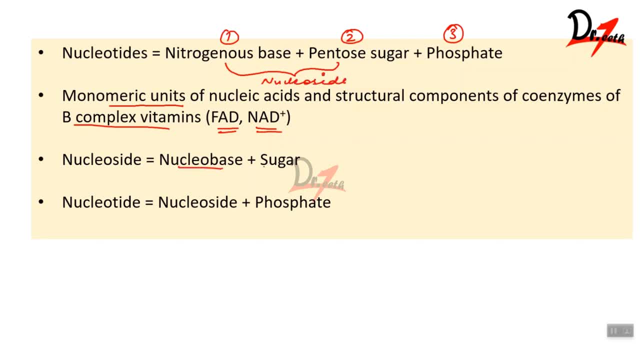 say it is the nucleoside, the nucleus base, and plus this sugar. now this nucleoside plus the phosphate nucleoside is the nucleoside and the phosphate nucleoside is the nucleoside, and the phosphate plus the phosphate together forms the nucleotide. for nucleotide we 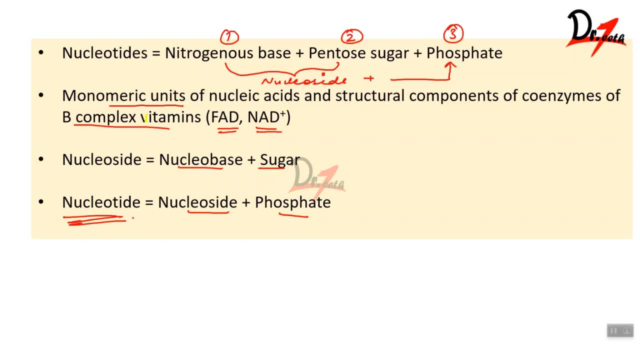 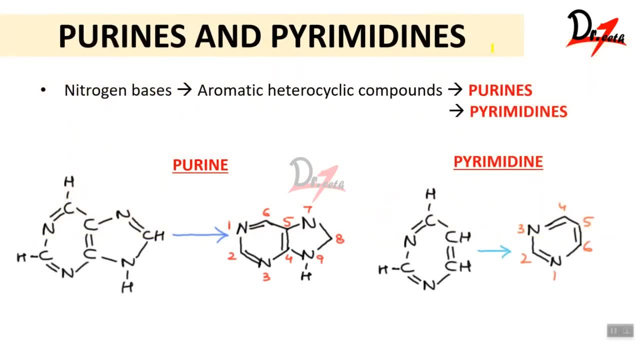 have the nitrogenous base, then we have the panto sugar and then we have the phosphate. okay, now moving on, let's talk about purines and pyrimidines. now, these are basically nitrogen bases, okay. what we studied, the nucleotides of compound, of the first component, is the nitrogenous bases, okay, in which we there. 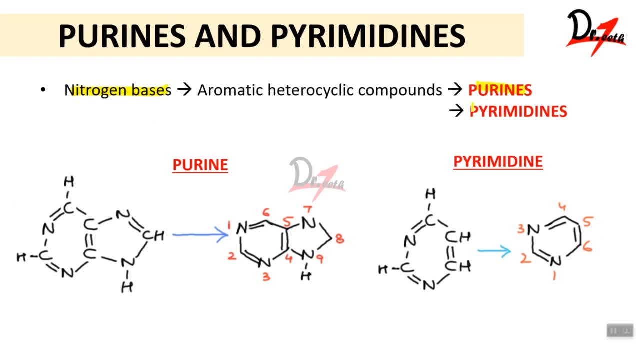 are two main components. we have producing the acts of purines and pyrimidines. okay, now, this is the example of purine and this is the example of pyrimidine. now, these are the aromatic heterocyclic compound, as you can see by the structure, 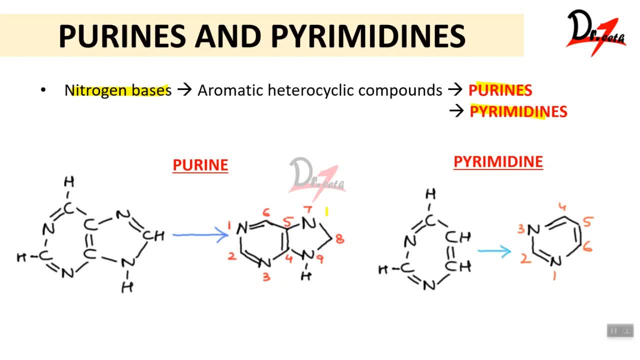 now one thing to notice with these compounds when we named the purines, okay, now these are numbered in anti-clockwise direction. this is the Anticlockwise Direction, which means one, two, two, d, equine, dot, three, four, Anthe, six, seven, eight, nine. 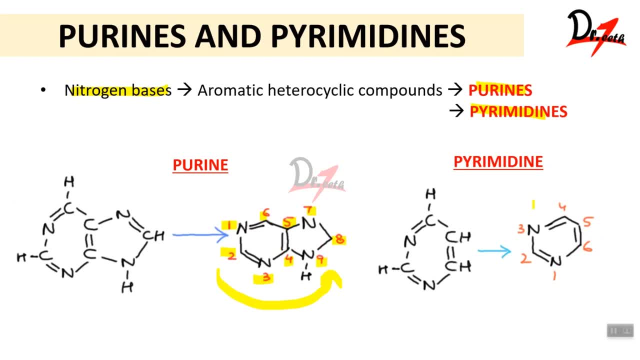 so. So this is the anti-clockwise direction, while for the pyrimidines these are numbered in the clockwise direction. like this direction, We have 1,, 2,, 3, 4,, 5, 6, okay, This is to be remembered. 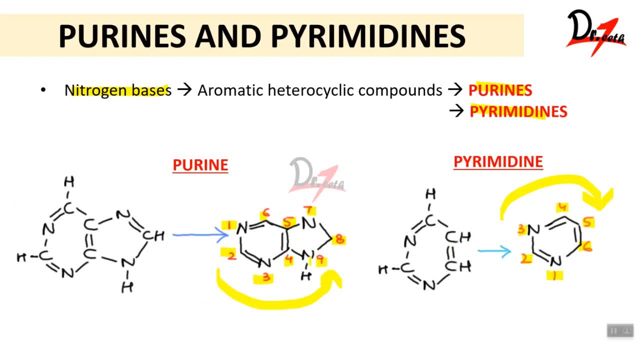 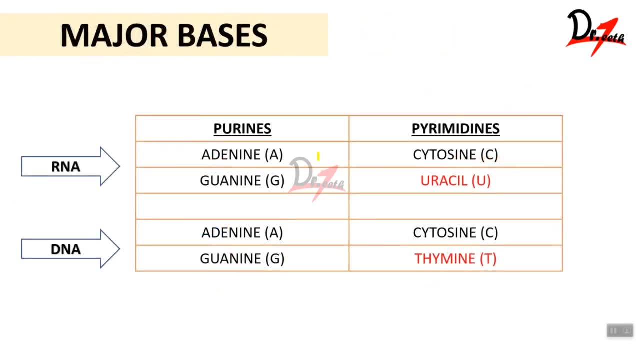 that the purines are numbered in the anti-clockwise direction and the pyrimidines are numbered in the clockwise direction. Now, moving on, what are the major bases For purines? we all know that there are 2 types of purines. We have adeninin and we have guanine. okay, And in DNA also. 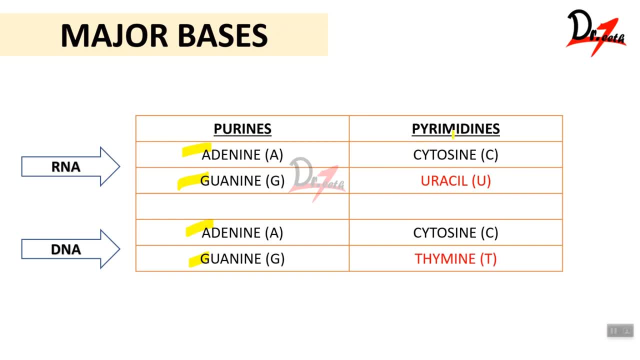 we have adeninin and guanine, And for pyrimidines we have. there are basically 3 types of pyrimidines: the cytosine, uracil and the thymine. Now, the only difference between RNA and DNA is 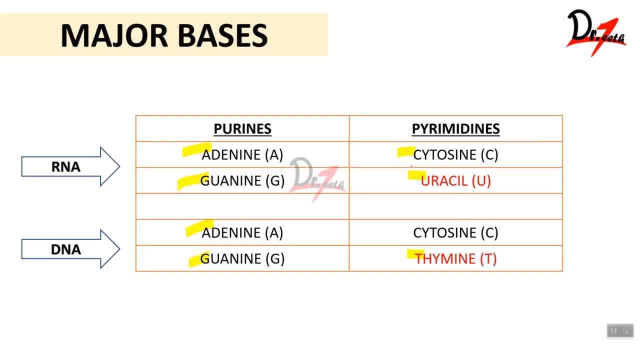 as you can see that in RNA we have the pyrimidine uracil, while in DNA we have the pyrimidine uracil. pyrimidine as thymine- okay, That is the only difference between the RNA and DNA. 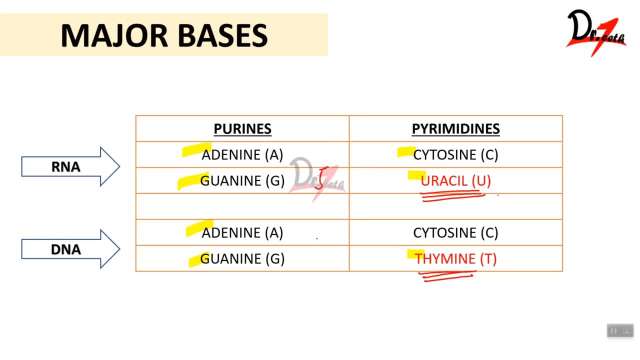 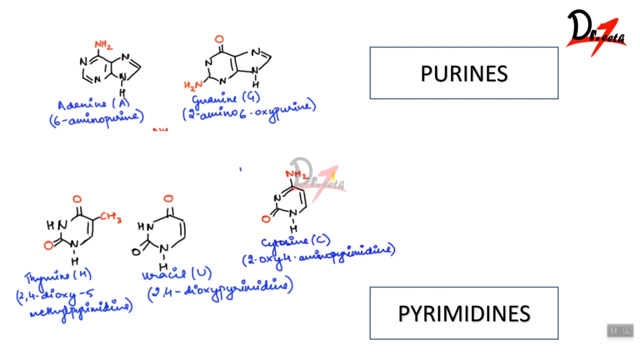 While the purines are same, we have adenine and guanine, and adenine and guanine here as well. Also, the cytosine is common in both of them. okay, Moving on, let's see them individually as structures. Now, coming on to first. we have the purines. okay, In purine. we studied that. 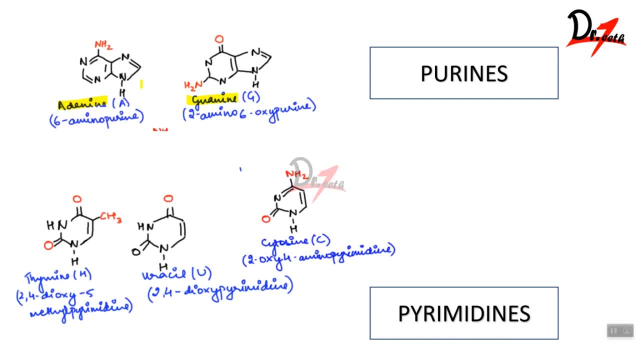 there is adenine and guanine. Now this is the structure Here. you can see that adenine is basically 6-aminopurine. okay, From the figure we can see 6-aminopurine. This is the amine group. 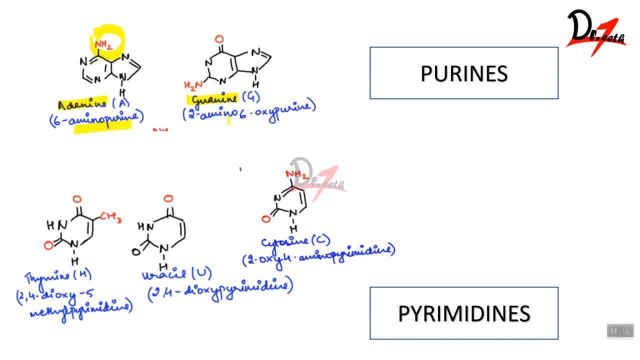 While in purines- the guanine one- we have 2-amino-6-oxypurine. Here you can see the aminogroup and here you can see the oxygen group. okay, One thing to make sure again is that the purines are. 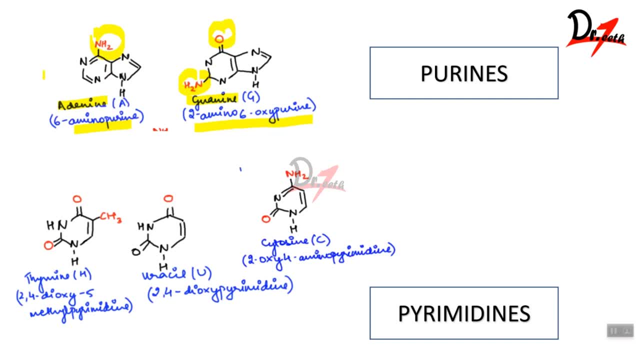 as we can see, numbered in the anticlockwise direction. okay, This is the anticlockwise direction, While the pyrimidines are numbered as in clockwise direction. Now let's look at the pyrimidines. We have thymine. okay, That is the 2,4-dioxi. This is 2,4-dioxi-5-methylpyrimidine. 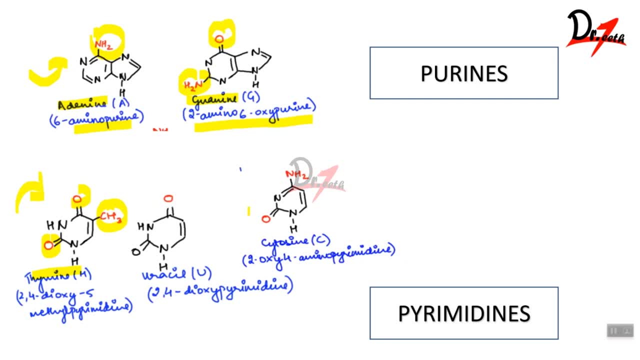 okay. So, basically, if either you can remember the structure and the name accordingly or, if not, you can remember the name and then remember, Remember the structure accordingly, okay. Then we have uracil, That is the 2,4-dioxi-pyrimidine. 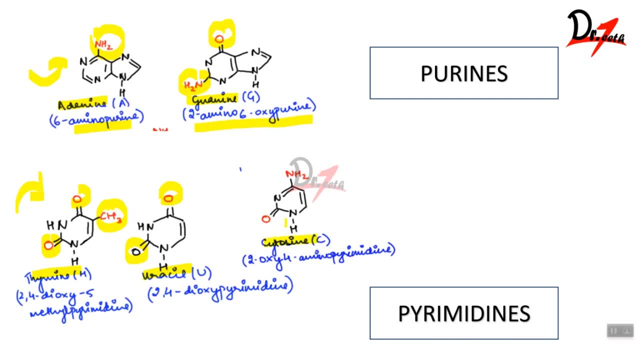 okay, Then we have cytosine. Cytosine is again 2-oxy-4-aminopyrimidine. okay, Now, one thing to see here is that the only difference between the thymine and uracil. 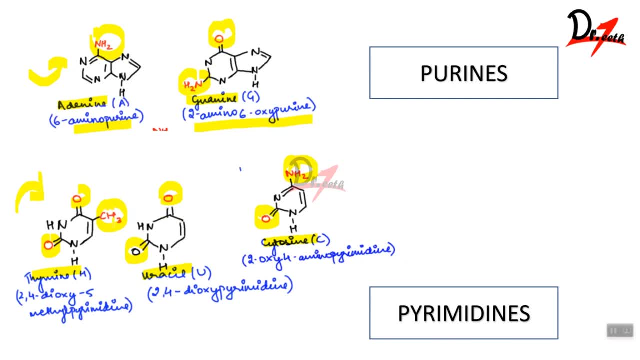 is the presence of methyl group in the thymine. You can see that the structure is actually almost similar In thymine. there is a presence of methyl group in the thymine. It is just the extra presence of methyl group, okay, Which is absent in uracil. So this thymine- 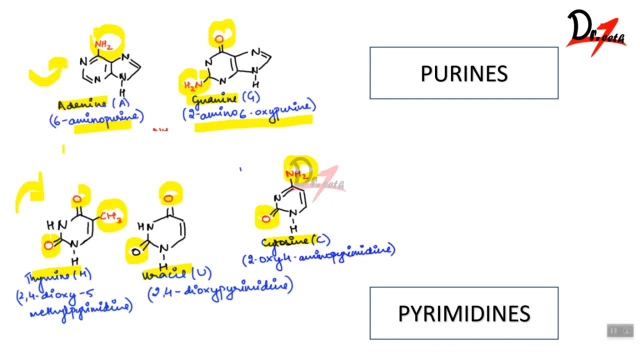 with the extra methyl group, is present, where we can see it in the thymine, we can see it in the DNA, and while uracil is found in the RNA. okay, I hope till now it is clear. Now, moving on, we have the tautomeric forms. Now, what is basically a tautomeric form? 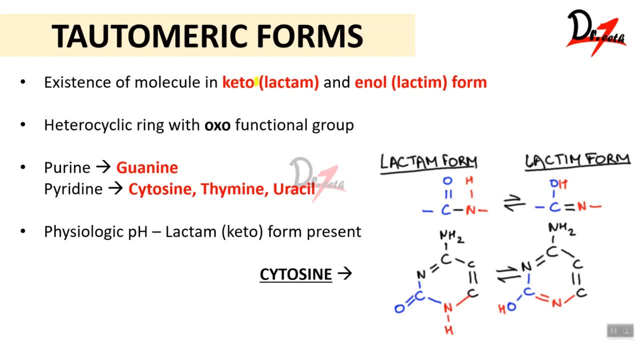 Tautomeric form is the existence of molecule in keto and enol group. We have the keto group that is known as the lactam and we have the enol group that is known as the lactam. okay, So these two basically coexist. Now we can see by keto. we all know that the keto group means. 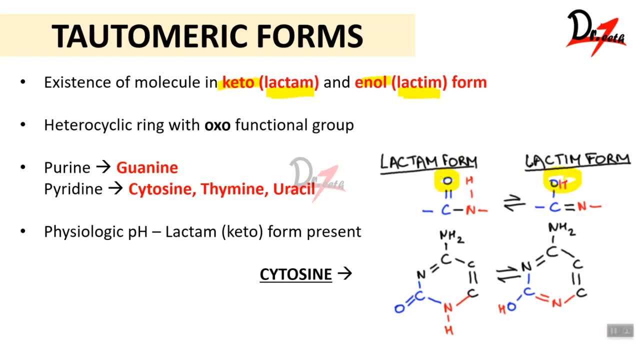 there is the oxygen, and by enol we means there is the OH group. okay, Now, here you can see the example of cytosine. This is the lactam form, or keto form, where there is a presence of oxygen, and in the enol form we have OH. okay, Now, this is basically a heterocyclic ring. 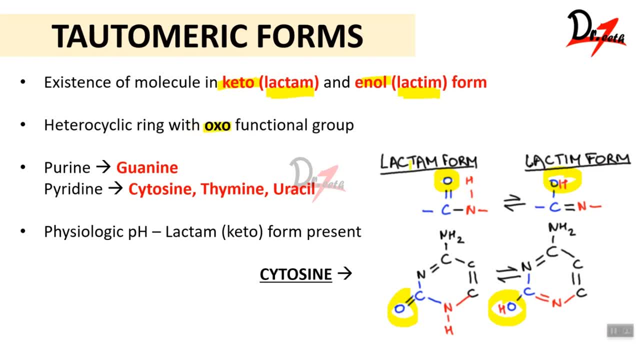 with oxo functional group By oxo. we all know that there is the presence of oxygen, okay. Now in purine, the guanine shows this tautomeric form, and pyrimidine, we have the cytosine thymine uracil, which means all three of them show the tautomeric forms, okay. So 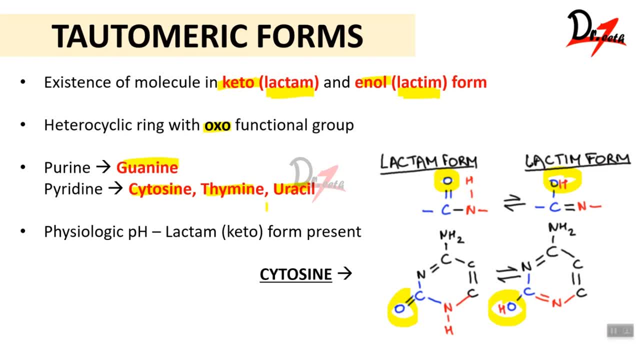 it is basically that in adenine, that is a purine, the tautomeric form is absent. rest others it is present, okay. So also one thing to notice here is that at the physiologic pH in the body the keto form is present, okay, Not the enol form. the keto form is present. Now moving on. 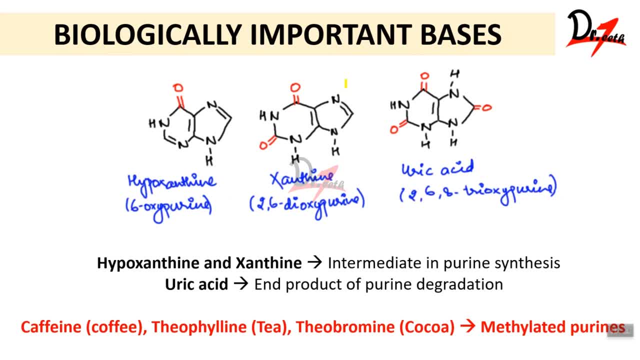 let us talk about some biologically important bases. okay, So we have the hypoxanthrope xanthine, we have the hypoxanthine, we have the xanthine and we have the uric acid. okay Now. 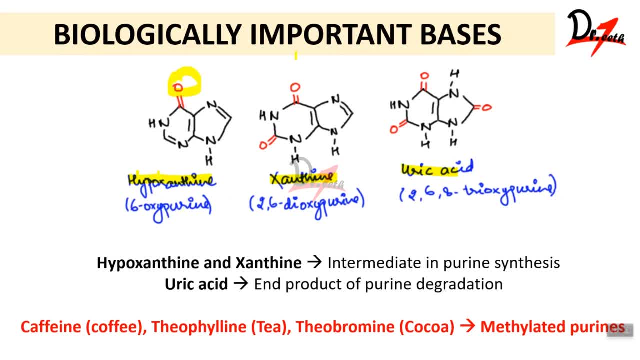 with the name, we can see 6-oxypurine. this is the oxygen group 2,6-dioxypurine, which means there are two oxygens present, and 2,6,8-ryoxypurine, which means there are three oxygens present. 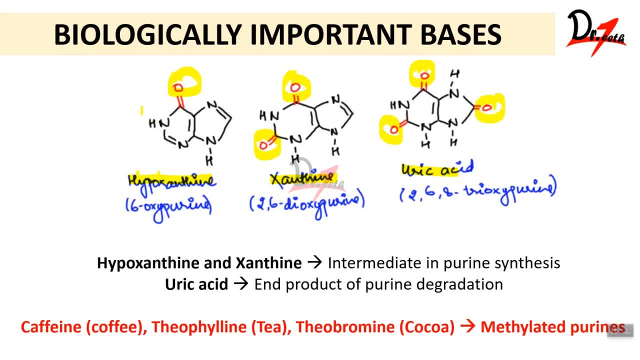 So you can see, the structure is almost the same. In first case we have one oxygen, in second case we have two oxygens and in third case we have three oxygens Now: hypoxanthine and xanthine. 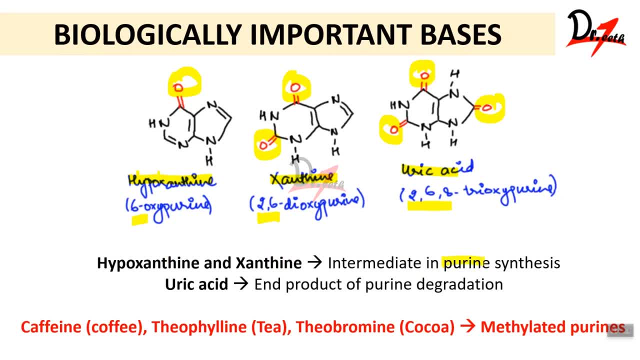 are basically intermediate in the purine synthesis, okay, While the uric acid is basically the end product of purine degradation. okay, And one exciting factor to know about here is the caffeine that all of us are so addicted to, or some of us are also addicted to the thee. 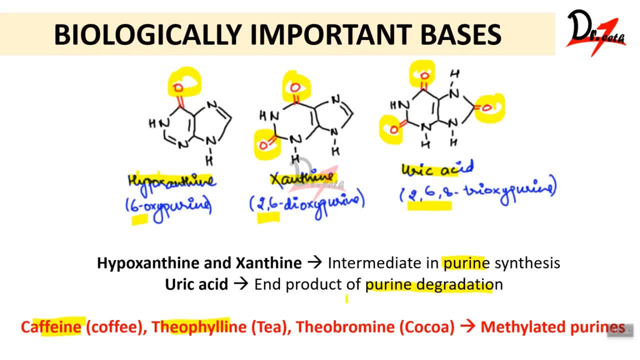 that is the theophylline, and we all know that pastries are our weakest point- that is the theobromine that is present in cocoa- are basically nothing but phthalated purines, So we can say that we are actually addicted to drinking or eating purines. 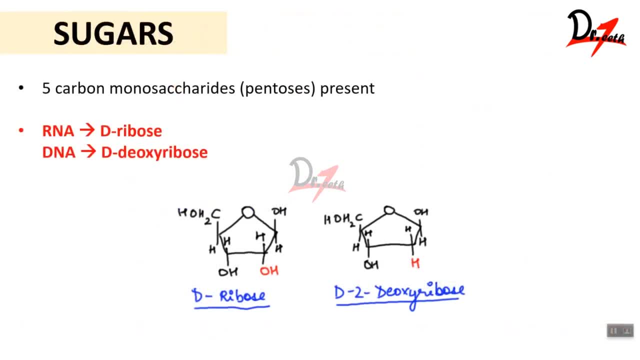 okay, So moving on, let's talk about sugars. Now we studied that the sugars are the second part of the nucleotides. okay, So in sugars we have 5-carbon monosaccharides, or we can see. 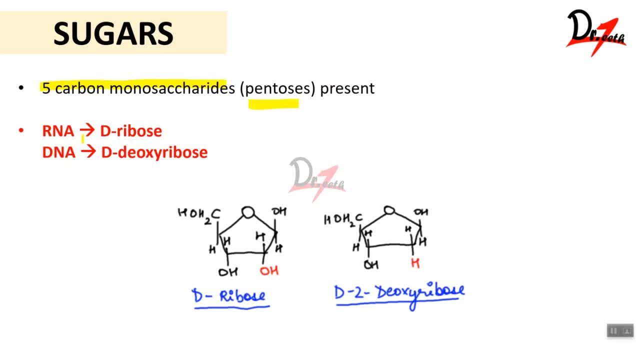 the pentosis present. okay, Now in pentosis. in RNA there is d-ribose- here you can see the d-ribose, okay. And in DNA we have the deoxyribose. Now, this is where the name for the DNA and RNA. 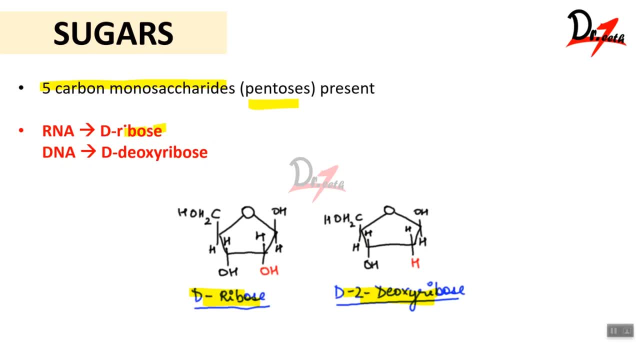 basically arrives from: In RNA, we have ribose, hence the name ribonucleic acid, and DNA, we have deoxyribose, and hence the name deoxyribonucleic acid. okay, So these are the structures Here. 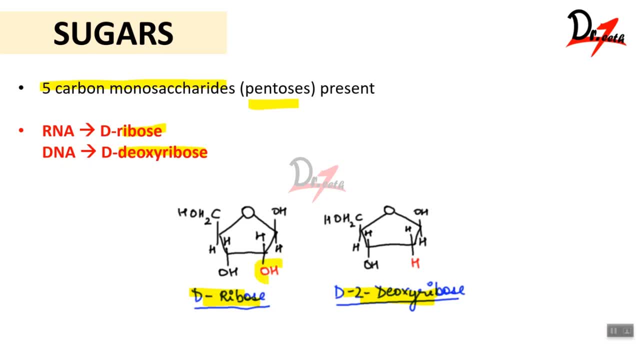 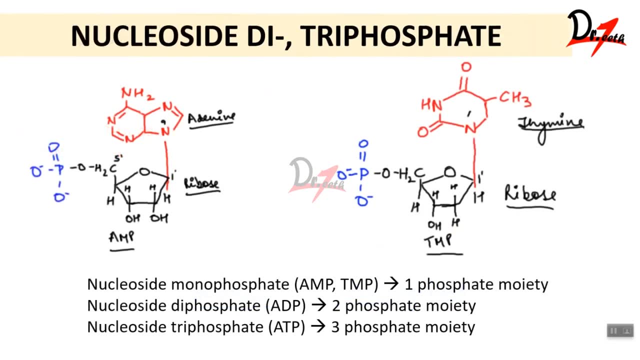 you can see, the major difference lies here. the ribose has OH, while the deoxyribose has H. okay, Moving on, let's talk about nucleosides. okay, The nucleosides, and basically the di and triphosphates. So how do these nucleosides combine? Now, we studied that nucleoside. 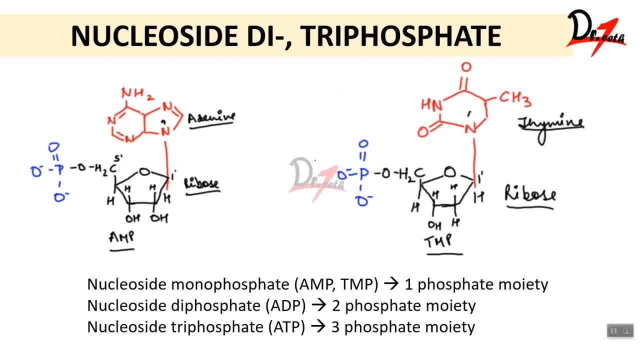 I hope you all remember that the nucleoside is nothing. but we have the nitrogenous base and plus we have the sugar which makes up the nucleoside. okay, So in adenine and ribose together form the nucleoside which is known as the AMP. okay, Here you can see these. 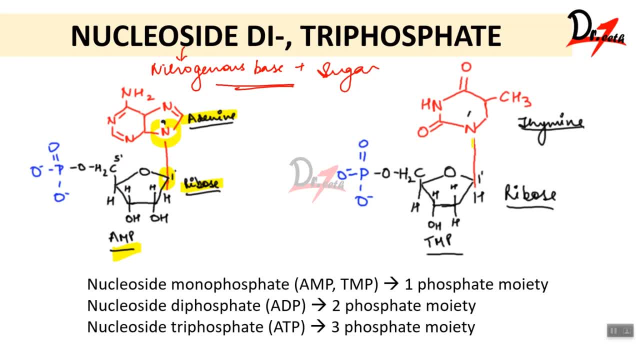 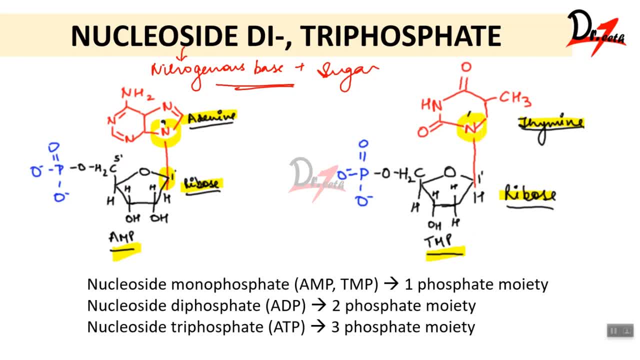 are the nucleosides. okay, Here you can see this is also connected with the same one. Now, the nucleoside monophosphate basically has one phosphate moiety, as you can see. one and one each, okay. So examples of nucleoside monophosphate is AMP and TMP. 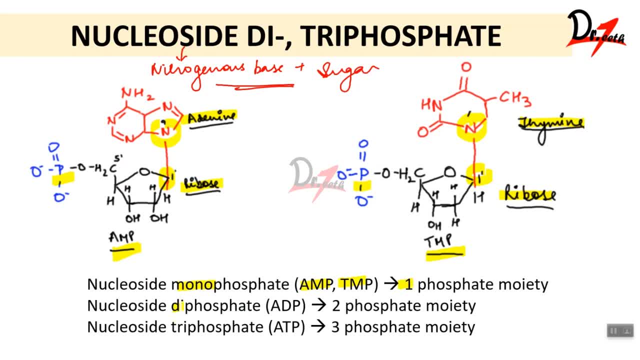 which has one phosphate moiety. Then in nucleoside diphosphate we have ADP, that has two phosphate moieties, and in nucleoside triphosphate, that is the ATP 3-phosphate moieties. now we all know that the ATP ADPs are nothing but the. 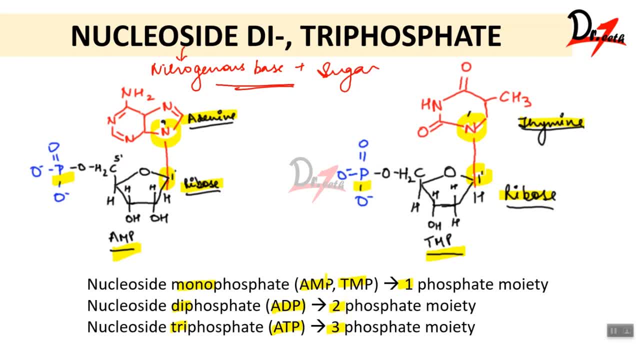 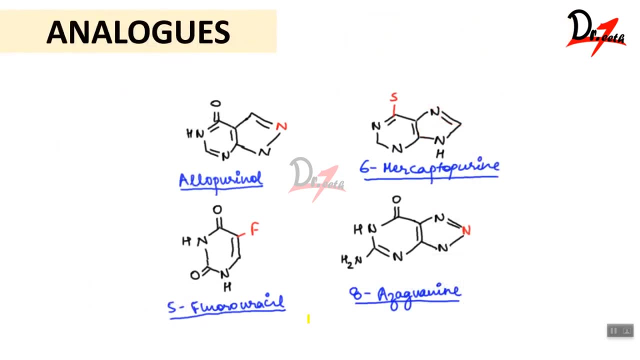 energy giving products. okay, so now you can remember: in AMP, TMP 1, in ADP 2- phosphates and in ATP 3- phosphates. okay, this is how you can remember: M means mono, D means di and T means tri. now these are basically the analogues, okay. 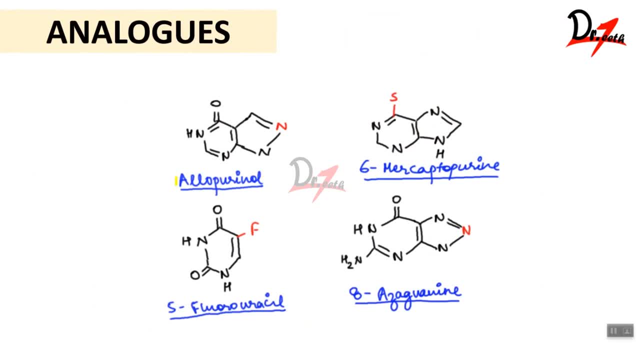 in analogues we have the allopurinol now. this allopurinol basically is used for treating hyperuricemia and gout. okay, the allopurinol is used in treating hyperuricemia and gout. this 6 meta-captopurine is used to treat cancer. 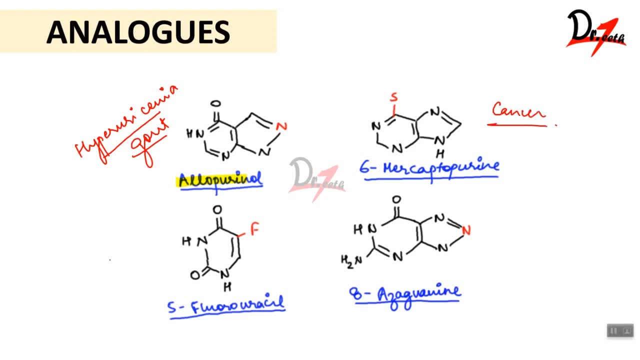 also these 5 meta-captopurine are used to treat cancer and these 5 meta-captopurine are used to treat cancer also. these 5 5-Fluorouracil is also used to treat cancer and 8-Azoguanine, as we can see here, treats the acute leukemia. 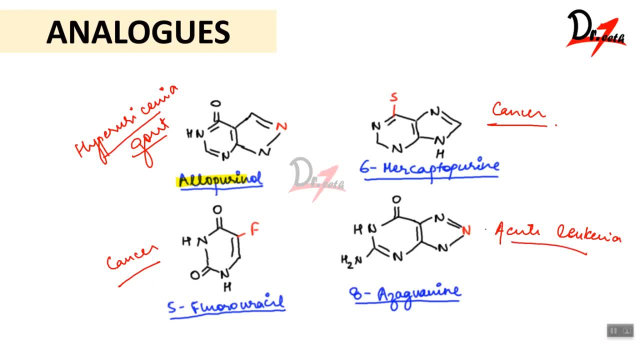 So these are some of the important analogs that we have to remember: The allopurinol is for hyperuremia and gout, The 6-Metacarpoputrine is for cancer, 8-Azoguanine is for acute leukemia and 5-Fluorouracil is the cancer. 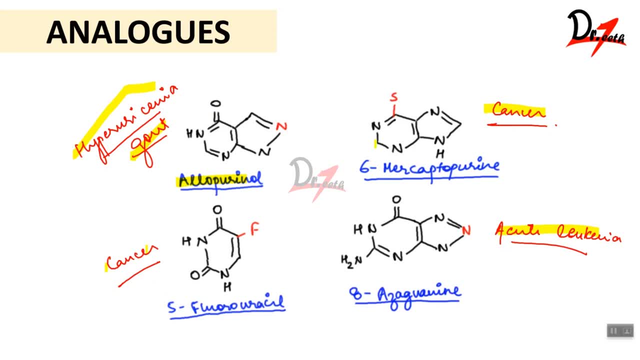 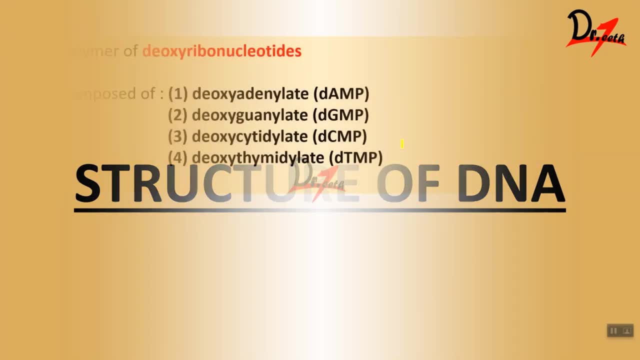 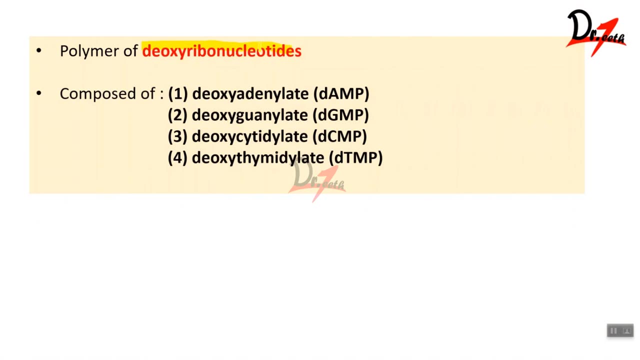 Now by the name. here you can also see and study the structures. Moving on, let's talk about the structure of DNA. Now, we all know that DNA is basically made up of deoxyribonucleotides, So it is basically composed of deoxyadenylate. 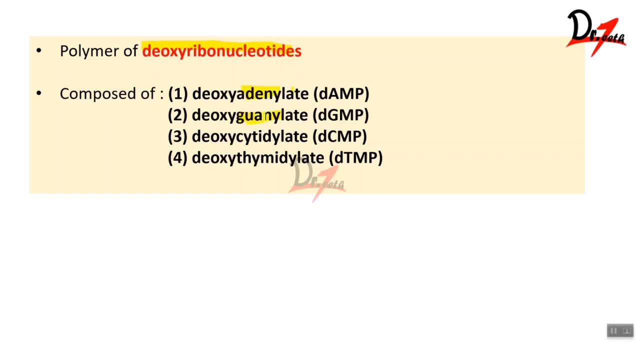 Deoxyguanylate, deoxycytidylate and deoxythymidylate. Now you don't have to mug up this. This is basically. we all studied before that the DNA is made up of adenine, guanine, cytosine. 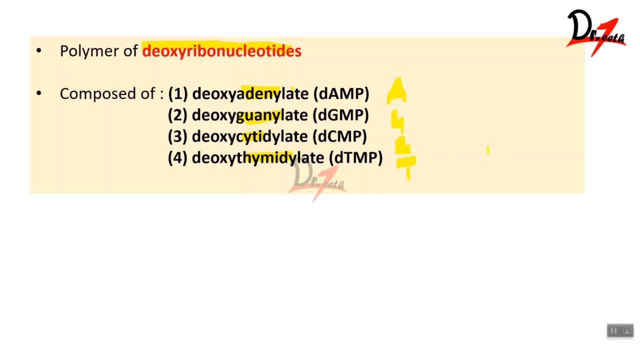 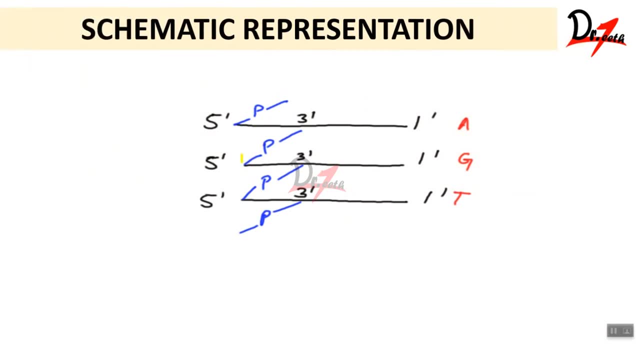 and thiamine. So this is just their names, So you can remember it this way. There is nothing hard and fast in this. Now, here you can see, this is the basically schema. This is the schematic representation of the DNA. So what we see here is just look. 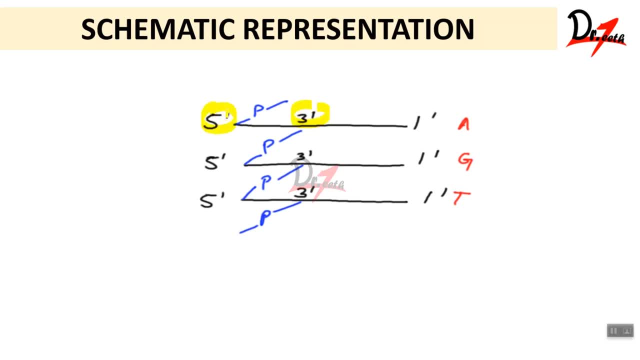 Now this is the 3 and 5 we can see here. This is the phosphodiester bridge. The 3 and 5 is the. where we can see the phosphate is the 3, 5 phosphodiester bridge, and this horizontal line that we see here basically shows the carbon chain of sugar with base. 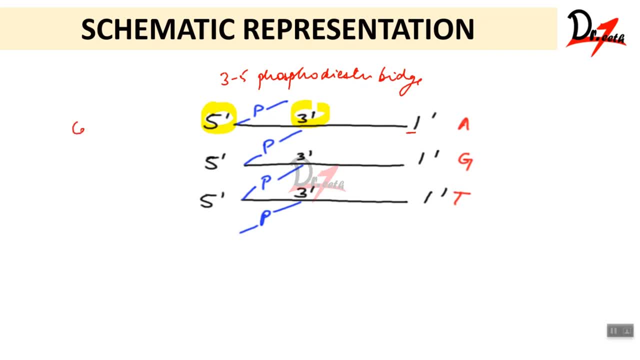 attached at C1.. Carbon chain of sugar. okay, Then the middle line, that is, the C3 phosphate linkage, is seen- C3 phosphate linkage- and the other end we can see there is a C5 phosphate linkage. Okay, So basically, in this schematic representation, this is the carbon chain sugar and you can. 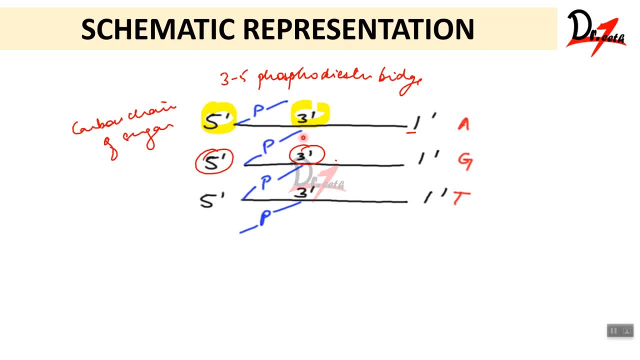 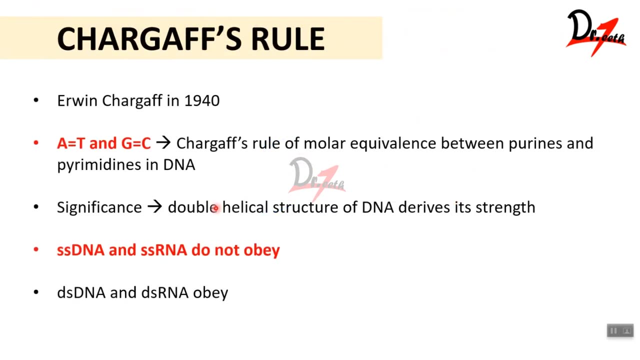 see the carbon chain sugar, which is connected by 3, 5 phosphodiester bridge. you can see, Okay, and one end is the C3 phosphate linkage and the other end is the 5 phosphate linkage. Now let's talk about charge Charge. 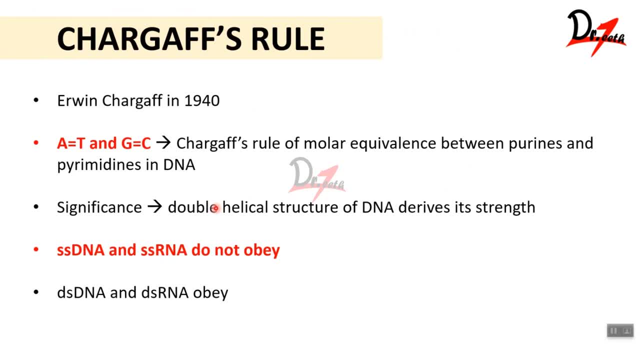 Charge. Charge. Now Eben Chargaff rule. Now Eben Chargaff in 1940 said that the A, T and the G? C that are in the equivalence of molar equivalent between Purines and Pyrimidines, which means that in DNA, whatever 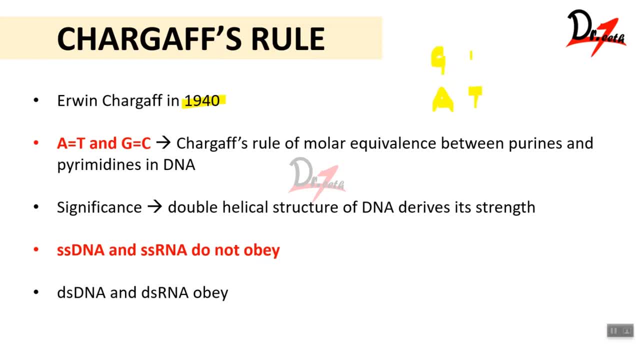 A will be, T will be the same amount And whatever C will be, G will be the same same, which means adenine will be equal to the amount of Thyme being present, guanine will be equal to the amount of cytosine present. okay, a chargers rule. 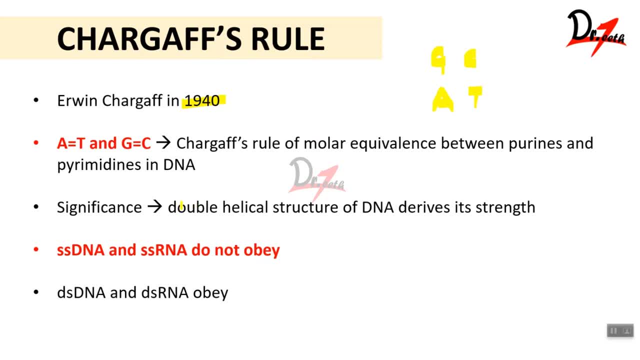 kata hai. ab iska significance kya hai? that the double helical structure of DNA derives its strength. just because these are equal, the DNA derives its strength from it. okay, and the important thing to note here is ki jo single structure, DNA, and the single stranded RNA jo hota hai, these do not obey the rule, only the 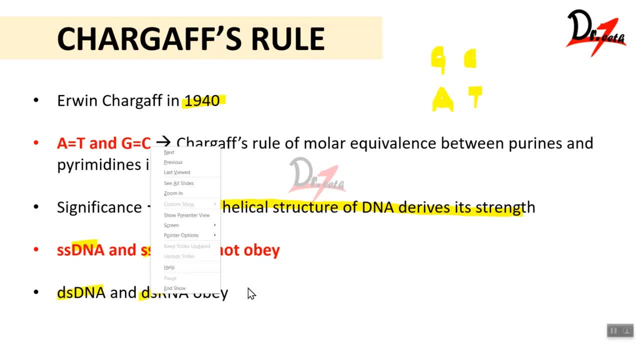 double stranded DNA and the double stranded RNA don't. if there is single stranded DNA, which means this is a single stranded DNA, either there can be guanine present or cytosine present. both of them cannot be present. okay, at the same time, ab aapki ek line mein, ek hi toh present ho sakta hai. they cannot be both of. 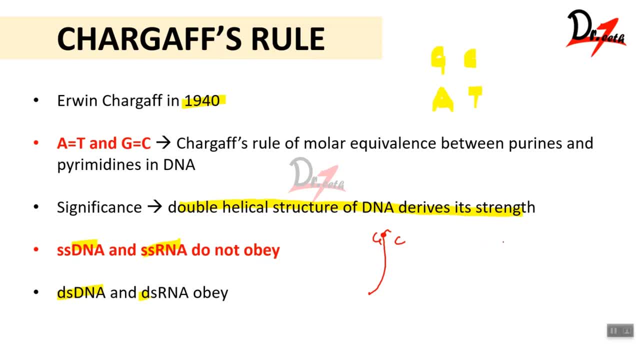 them present, but at the same time if these are double stranded, which means we have two strands here, so one strand has guanine and the other strand has cytosine. on the other hand, one strand has adenine and one strand has thymine. so what it? 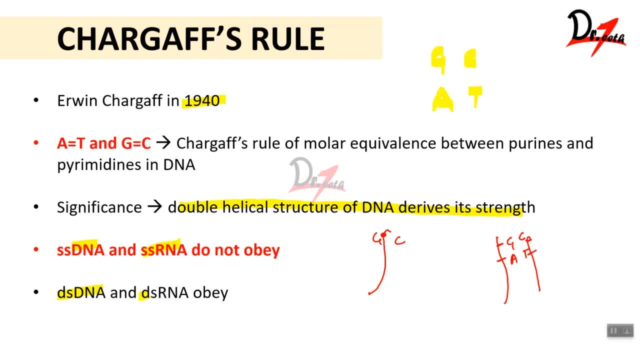 means is ki jitne bhi hongi. these will be equal, which means G will be equal to C and A will be equal to T. okay, there is no rule ki jitne GC hongi utne AT hongi. no, this is no such rule. but jitne G hongi, utne C hongi, aur jitna A hoga utna T hoga. 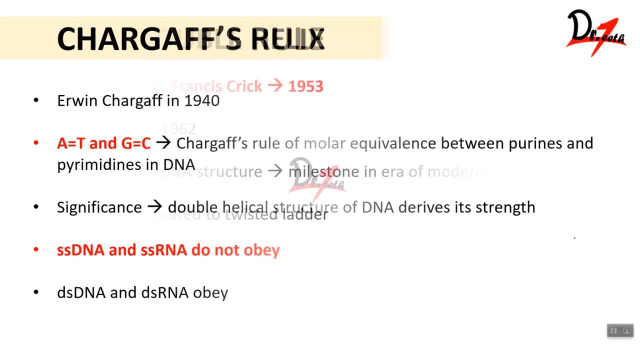 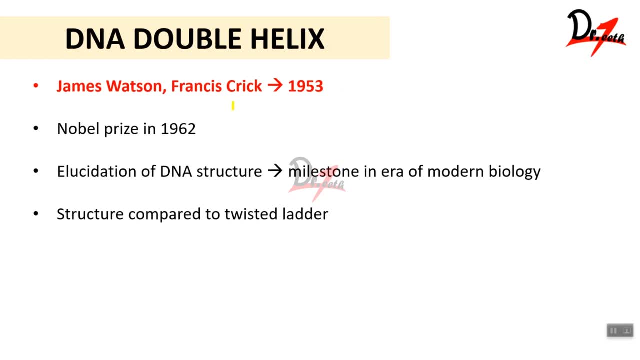 this is what the chargers rule says. now, moving on to the next rule, which is the moving on. we all know that there was another structure that was known as the double helix- okay, DNA, double helix. now, it was given by James Watson and Francis Crick in the year 1953. they both also won the Nobel Prize in the year 1962 for. 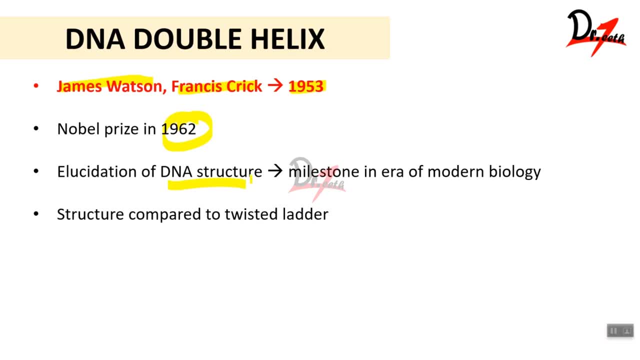 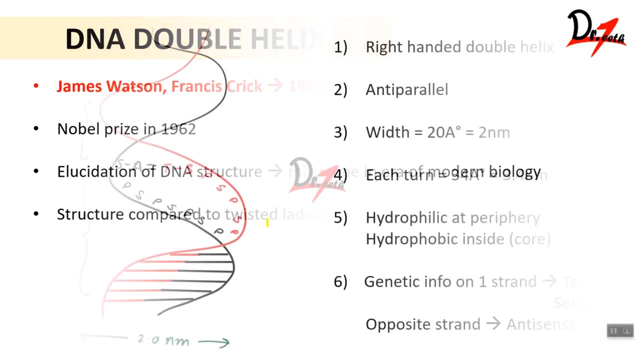 the same. you see, dation of DNA structure is basically considered as a milestone in era, which means that their DNA double helix was so powerful that it was considered as a milestone in modern biology. now this structure is basically compared to twisted ladder. let's see. now, here we 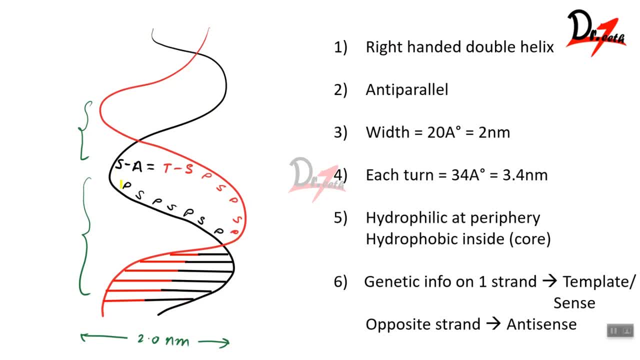 can see that this is the double stranded DNA structure. one strand is this one strand? is this okay now? what are the rules that we need to remember, or what are the features of DNA double helix? first, this is a right-handed double helix. okay now. the DNA double helix that they defined was right-handed. another thing to notice is: 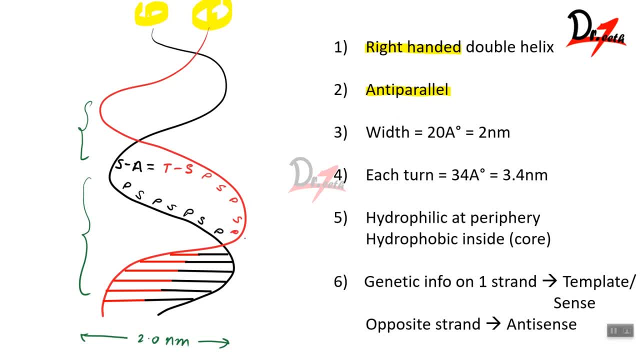 these are antiparallel, which means if this one is three to the black, one is three to five, like three to five linkage, then this one would be three to five linkage in an antiparallel direction. okay, which means if this starts as a three, 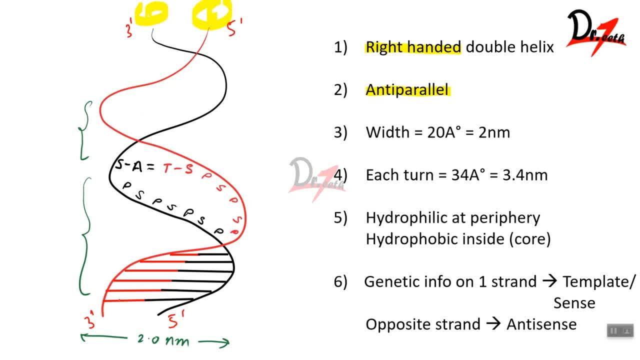 to five phosphodiester linkage now. so this will be opposite, that is, three to five phosphodiester linkage, okay, and their width would be somewhere equal to 2nm, or we can say 20 Armstrong, and each turn will have 3.4 nanometers. 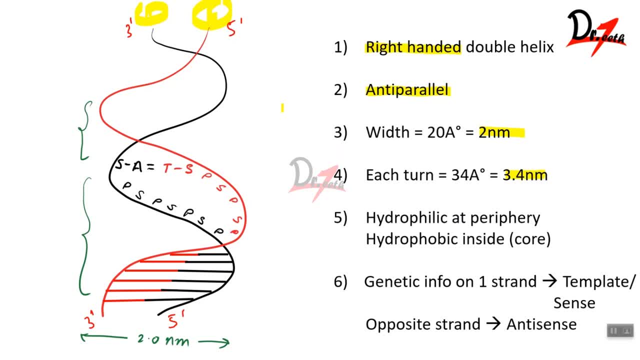 okay, which means each turn, as we can see here. from here, this is 1 turn. this is 1 turn. ok, now this is 3.4 nanometers and width, which means from here to here. we can see, here is two macros: iertes nanometers. ok, now hydrophilic at periphery. now, these are hydrophilic at. 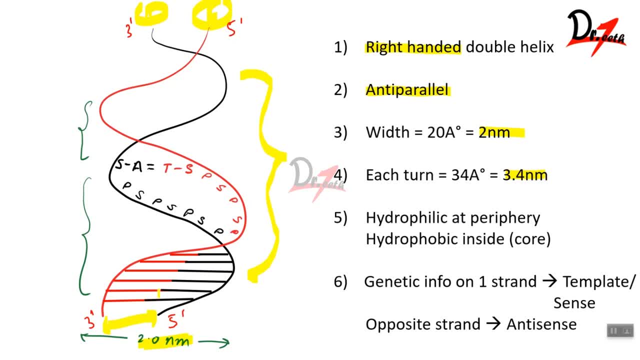 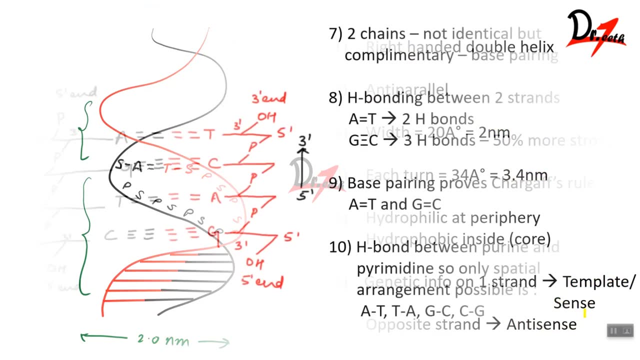 the periphery, but they are hydrophobic inside, which means at the core they are hydrophobic. ok now, one thing. another to notice is that one of them is known as the template strand, or the sense strand, and the opposite strand is known as the antisense strand, so which means that there are two chains present. ok now, 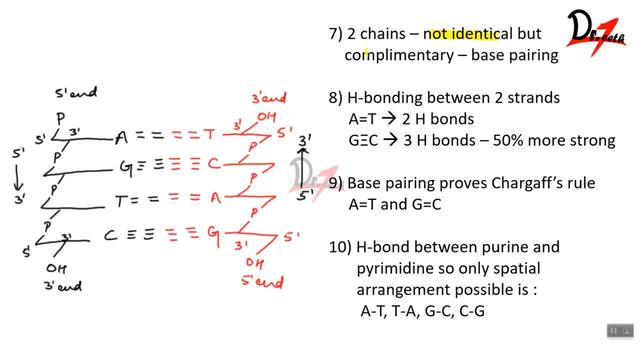 these two chains are not identical but complementary. there is complementary base pairing now, by complementary base pairing, as I earlier told you, that there will be adenine at one pair and thymine at the other, guanine at one and cytosine at the other. ok, this is how they pair. 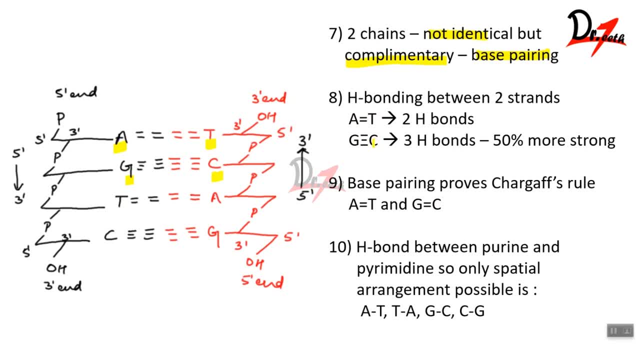 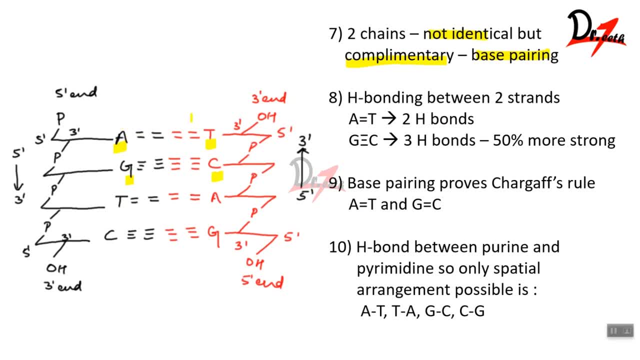 twin. the first one that we have. that is A and T. ok, these have two hydrogen bonds between them- that is why we denote it as A- T. and the guanine and cytosine, on the other hand, has three hydrogen bonds. okay, now we all know that. more the 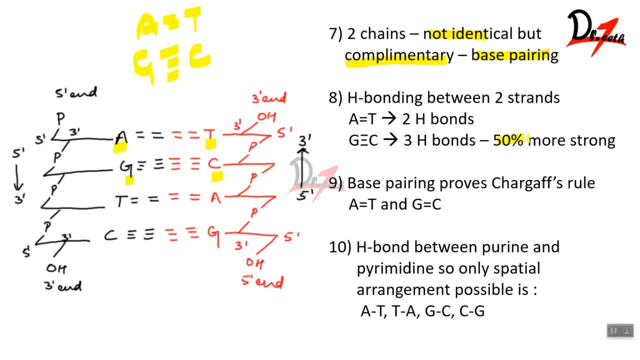 bonding there is, the more strong they will be. so these are 50% more strong. now let's come to the base pairing. ok now, one thing to be noted here was that the chargers rule actually applied here. ok, this was a proof that charges rule was. 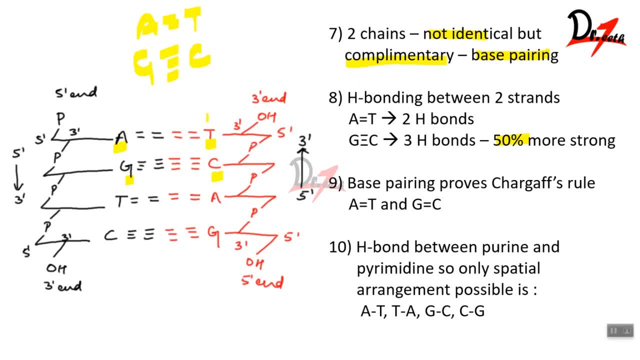 right, which means that the number of a's are equal to Ts, which means they are twins. heaiderman's rules words alone, which means they're twins, it is proved. and G equal to C's, which again tries to でしゃ Jew speaker的这个 virtue. that means the number of A 맞아 T across the personas就是. 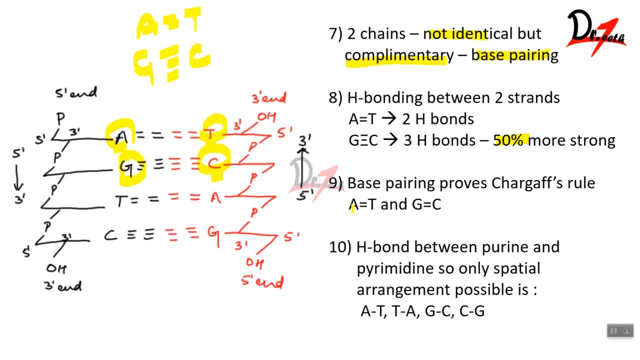 proves it that they are twins. okay, Now, this is for your understanding. only, they are not actually twins. Now, the H bond between purine and pyrimidine was only possible in spatula arrangement. Now, here you can see. we also talked about. you know how 5, 1 is. 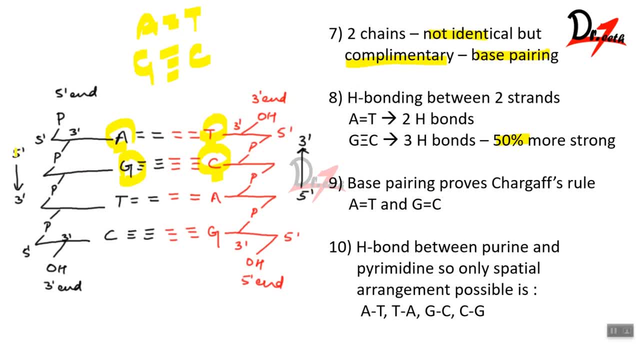 the anti-parallel one, and then 1 is the parallel one, which means 1 starts from 5 to 3, then the other one has to start from 3 to 5, okay, Now let's talk about the confirmations, okay. 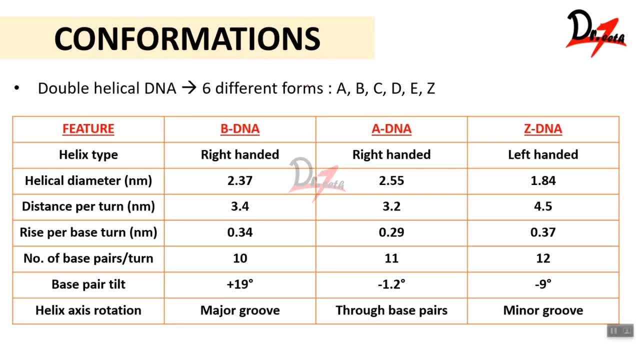 So by confirmations we mean that these double helical DNAs are basically present in 6 forms: A, B, C, D, E and Z. okay, And one thing to notice: that A, B and Z are the important ones. 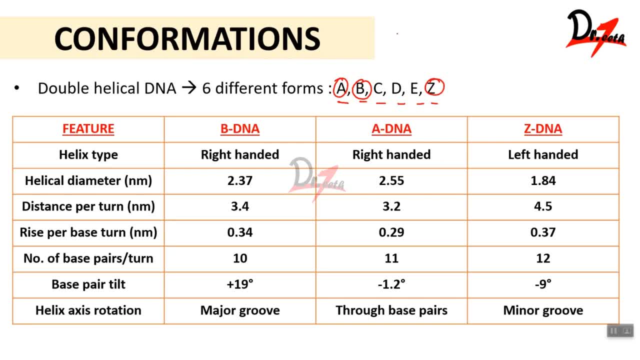 that we need to study And the B form. now B form was basically 1,, 2,, 3,, 4,, 5,, 6,, 7,, 8,, 9,, 10,, 11,, 12,, 13,, 14,, 15,, 16,, 17,, 18,, 19,, 20,, 21,, 22,, 23,, 24,, 25,. 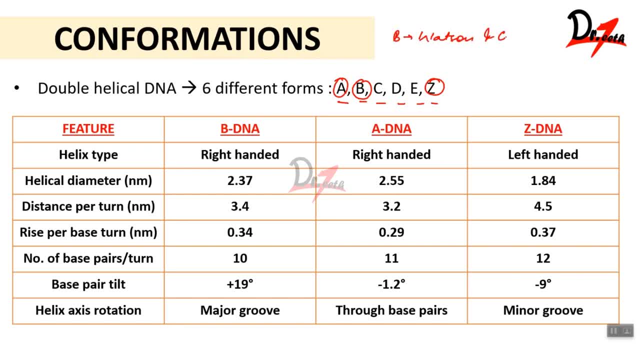 what the Watson and Crick model told us. Watson and Crick model told us: okay, That is, it is the most predominant form. it is the most predominant form, And by most predominant form we mean that at physiological pH in our body, this is the most predominant form. 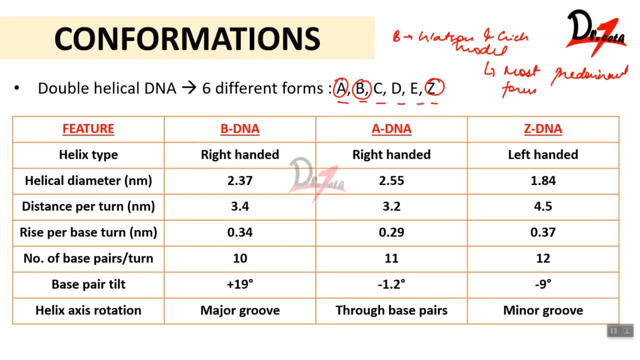 So now let's look at them. Now we all know that B and A DNA are right-handed, while the Z DNA is left-handed. The helical diameters are 2.37,, 2.55, 1.84.. Distance per turn: as we studied in. 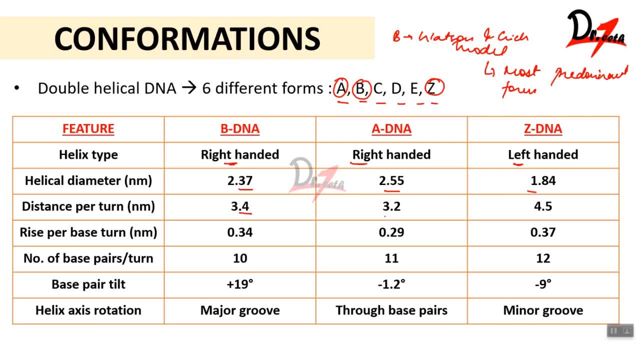 Watson and Crick model is 3.4.. The A DNA has 3.2,, while the Z DNA has 4.5.. Rise per base turn: we have 0.34 nanometer for the B DNA, 0.29 for A and 0.37 for Z. Number of base turns is 10.. 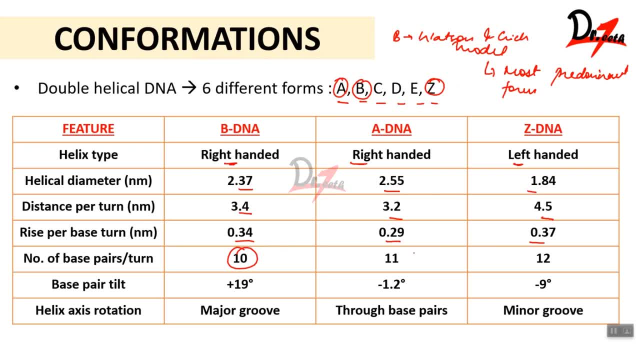 That means that there are 10 bases present In one turn. for A DNA, we have 11,, for Z, we have 12.. And the base pair tilt is 19 degree- here it is minus 1.2 degree and here it is minus 9 degree, And the helix axis rotation is at major. 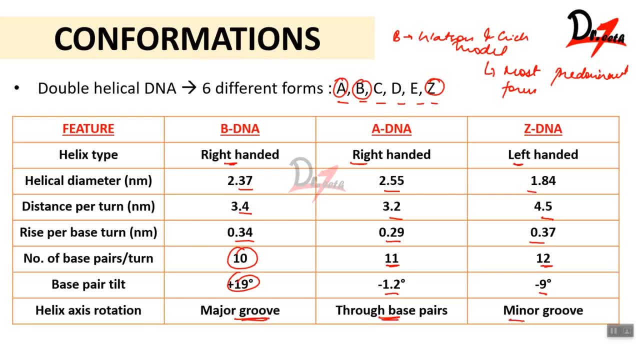 groove, here through base pairs and here through minor groove. Now we don't have to literally mug this up or anything, but the most important one here is B DNA. So even if you remember B DNA and all the properties, it's all right. But all the B DNA properties, it's all right, But all the B DNA. 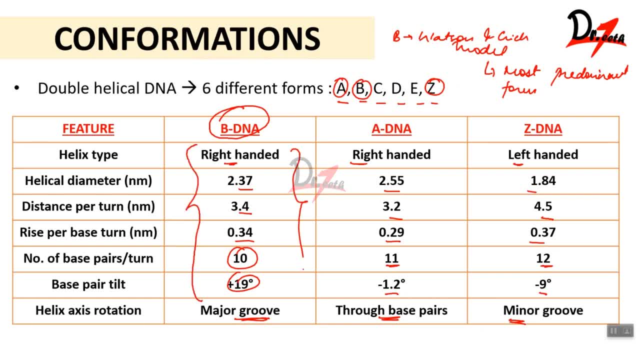 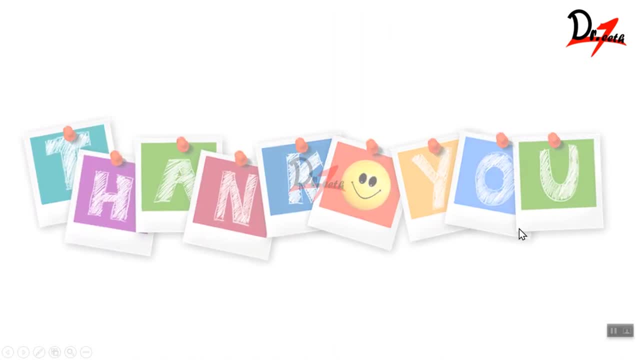 things. all the features of the B DNA are important ones, okay, Because this is what the Watson and Crick model told us about, And this is the one thing to remember is this is the most predominant form, okay, So thank you all. This was all for today. I hope you understood something out of it. 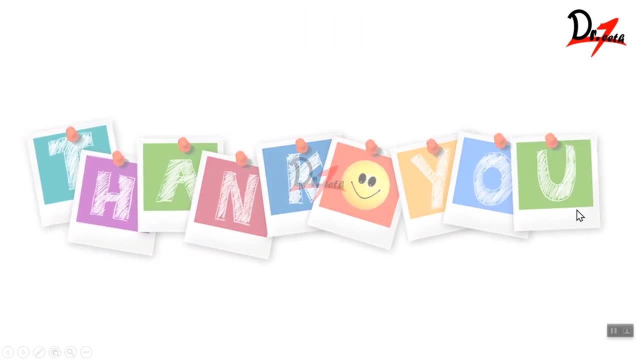 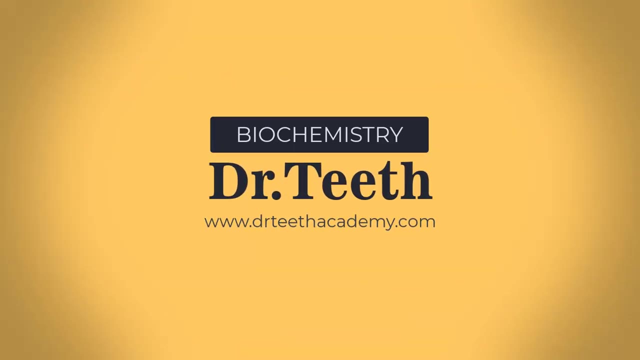 Thank you so much And I'll be seeing you in the next video And we'll talk about further more about DNA in the next video. Thank you, Thank you.